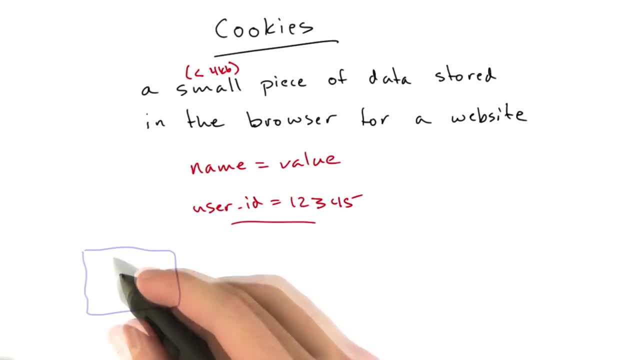 5. So to kind of draw you a little picture of how these things fit together, you know we might have your browser and it makes requests, you know, to some web servers And the web server might send back in its response some cookie. 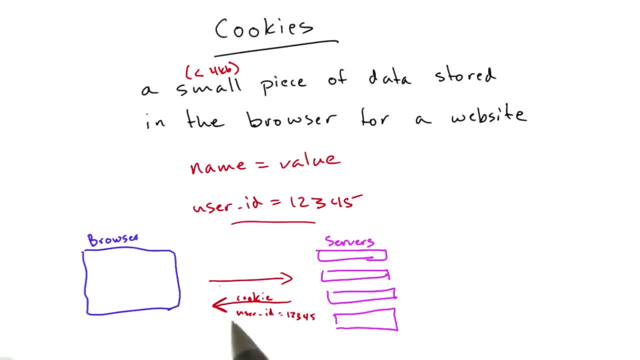 data, And this is in the form of an HTTP header, And then your browser basically just stores this cookie. It's associated with this website- We'll talk more about that shortly- And then every time your browser makes a request to this website in the future, now that it has this cookie, it will. it will. 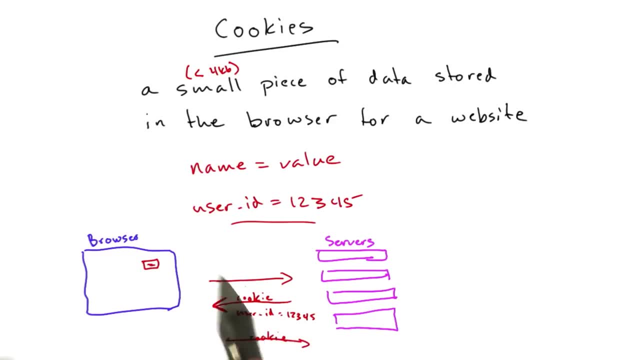 send the cookie back to the server. So you know if you're logging in, you know you might. you might post some form here And the server might respond with. okay, you know, welcome to our website. you're user 1,, 2,, 3,, 4,, 5. And. 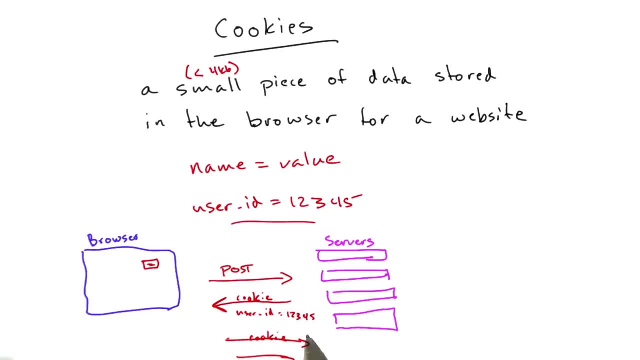 then on every future request you say: hey, I'm user 1,, 2,, 3,, 4,, 5.. And that's how the website knows that you're logged in. And a cookie, you know it's it's. it's just basically a file that your browser 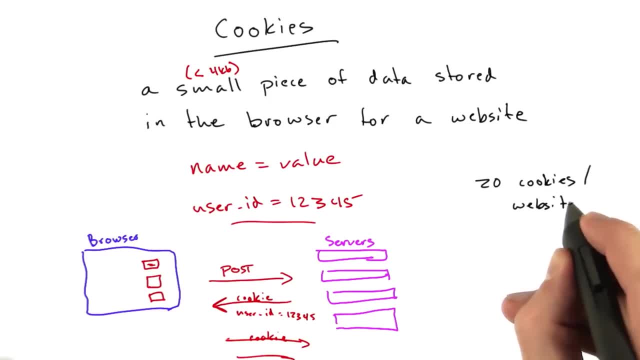 stores. Generally, you can store about about 20 cookies per website. Now, this is basically up to the browser. It's some sort of it. it it's a browser limitation. Another limitation is probably the length of the cookie. 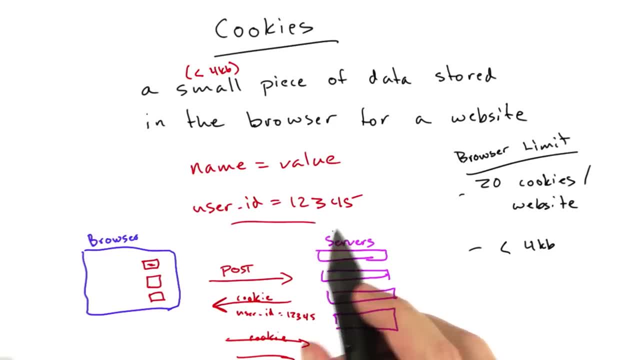 which we said is less than 4K, But in reality, you know, this is, this is five bytes, And we're probably, you know, most of the cookies you're going to be storing are, are not, you know, thousands of bytes. Another limitation is: 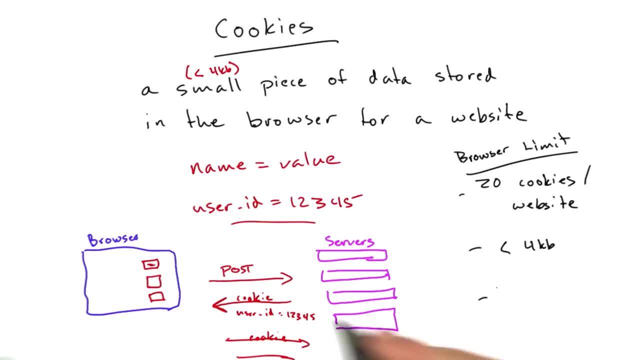 a cookie has to be associated with a particular domain. So you know a a cookie for udacitycom is only sent to udacitycom, And and udacitycom can only set cookies for udacitycom. So it's each. 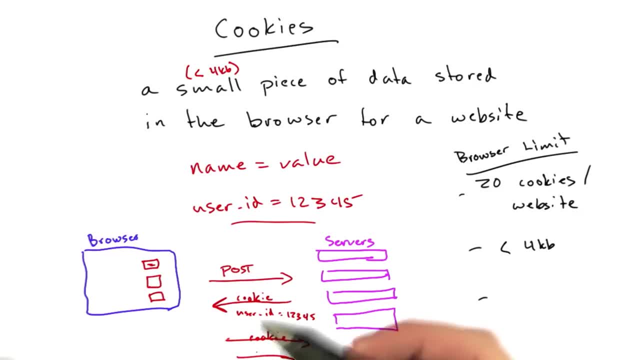 website has, you know, a few cookies that it can store that are private to that website. A lot of this depends on the browser to behave properly. So you know this: 20 cookies per website. that's an old Internet Explorer limitation. 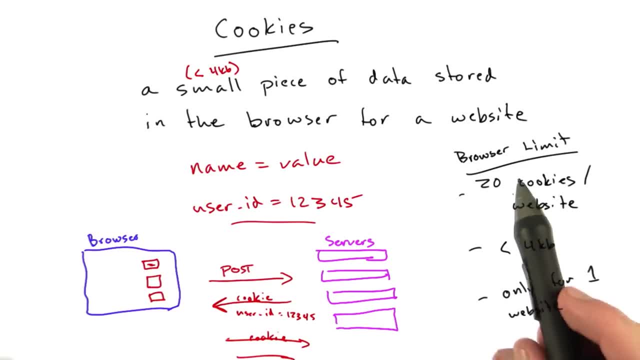 Honestly, I don't know what the limit is for modern browsers, But if you're storing more than 20 cookies on on a particular domain, you could probably rethink things a little bit. You know, maybe store more data in. you know a a. 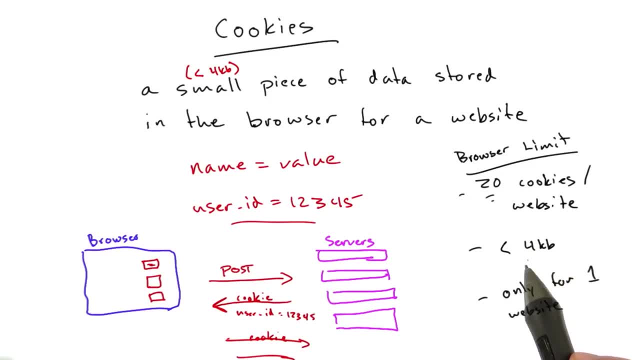 single cookie, The four kilobytes, again there's. there's so many things that can go wrong when you start sending big cookies that are, you know, 4,000 bytes long. You know you can set some.